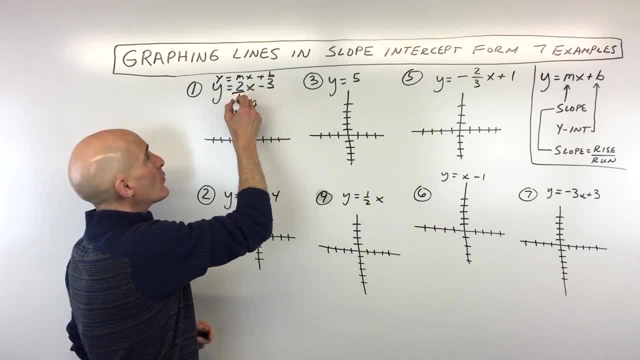 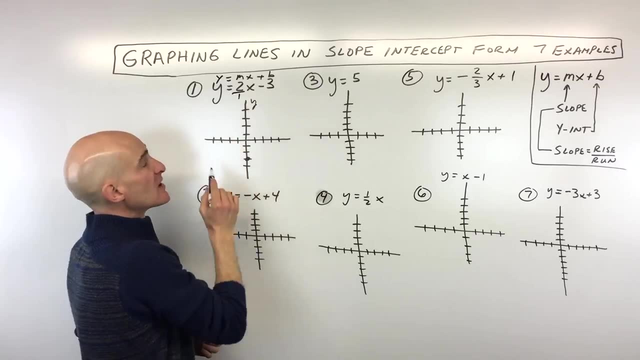 in this case, you see, we have a whole number 2.. You can write any whole number as a fraction by putting it over 1, because anything divided by 1 is itself right. So now when we look at it, we can see 2 is the rise and 1 is the run. So from this point- okay, not from the 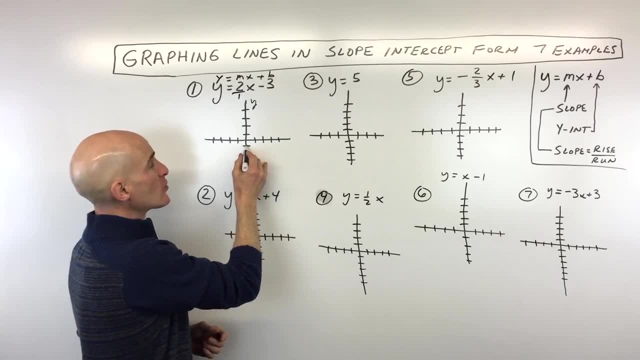 origin. but from this point we're going to rise 2, so positive 2, we're going up, run 1,. positive 1, we're going to the right and we've got another point on our line. Now you can repeat that process. 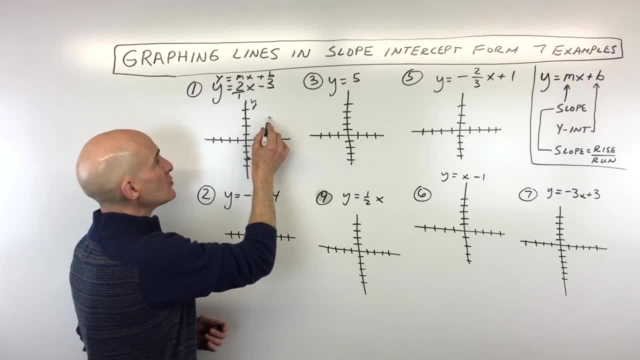 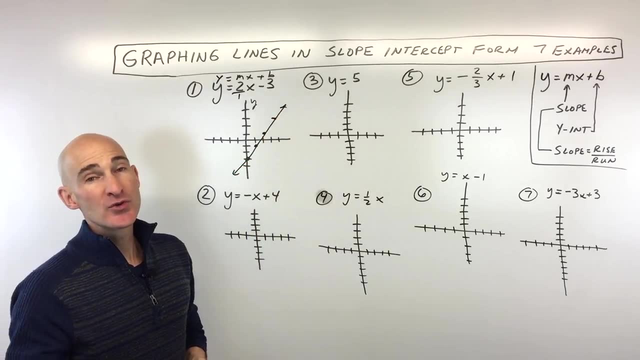 Rise 2,, run 1,. rise 2,, run 1, and that'll help you to get a pretty good graph of your line right there. Okay, let's do another example and you'll start to get the hang of this. 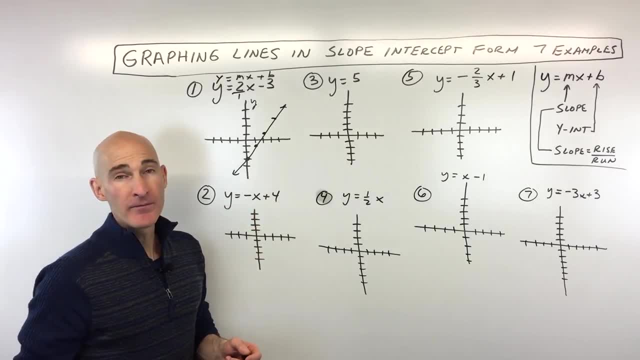 So number 2, we've got: y equals negative, x plus 4.. Okay, so now on this one, you can see that the y-intercept, the b value, this constant, is positive, 4.. Now remember, positive you go up, negative you go down, and we're on the y-axis, okay, so up and down, So up. 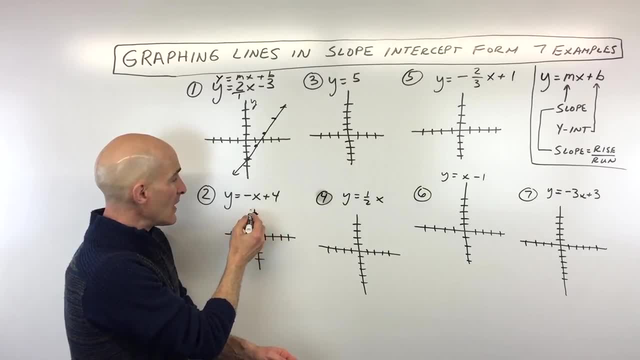 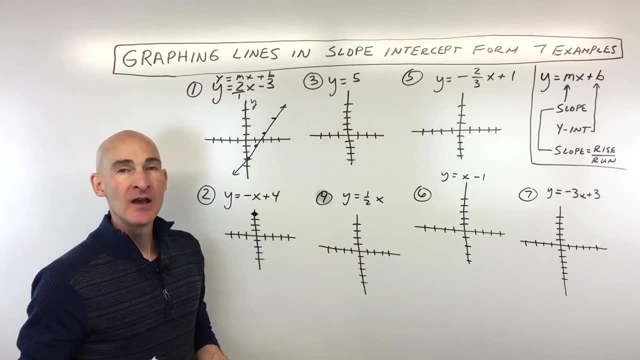 4,, 1,, 2,, 3, 4.. Right there, okay. and then now we have to find the slope. Now, remember, the slope is a number in front of, which means to the left of the variable x. Now, in this case, we just 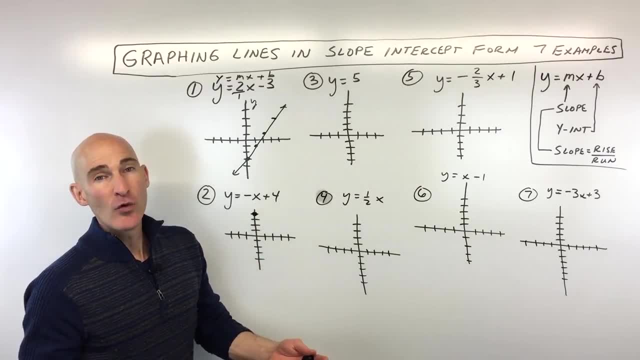 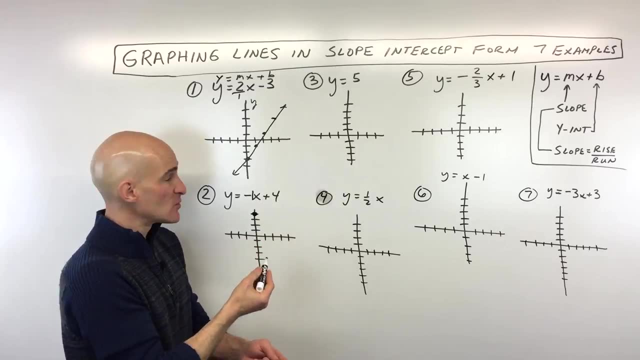 see a minus sign here. What does that minus sign mean? Well, it means negative 1, right, So negative 1, I'm going to put that in there like that, because 1 times anything is itself right: 1x. negative x is the same as 1x, and then negative 1, we can also make into a fraction. 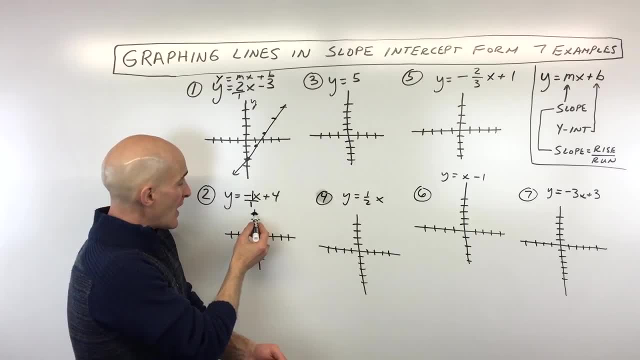 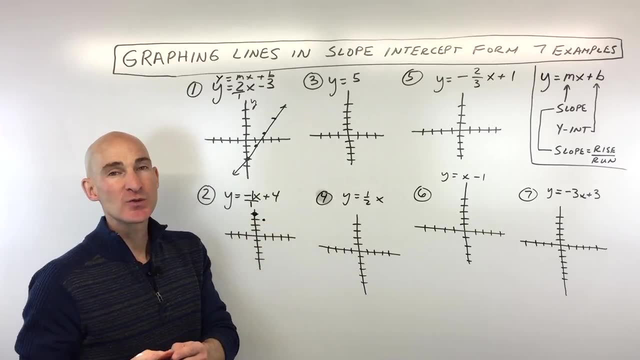 by putting it over 1, so negative 1 over 1.. So now what I'm going to do is, from this point, 1, right 1.. Okay, now some students get confused because what they think is, they say: well, 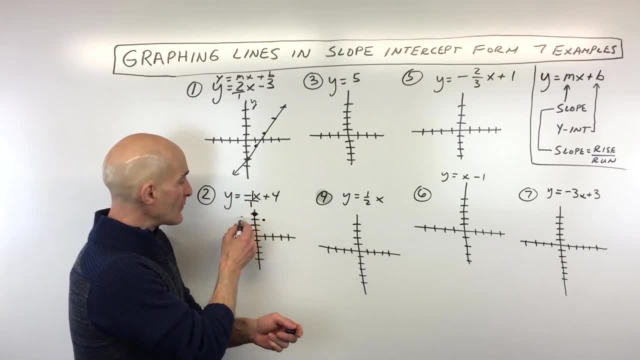 Mario, you know negative 1 over 1, like you went down 1, how come you didn't go left 1?? Well, here's the thing, remember when you're going up that's positive, down that's negative. 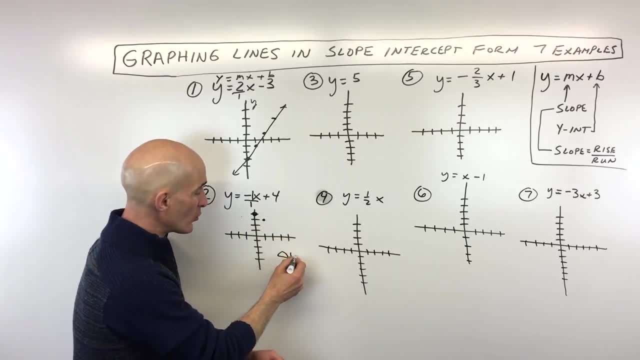 right that's positive, left that's negative. and we're looking at the slope, we're looking at the change in y over the change in x, right. So this negative 1 means that I'm going down 1, okay. and then this positive 1 means I'm going right 1.. 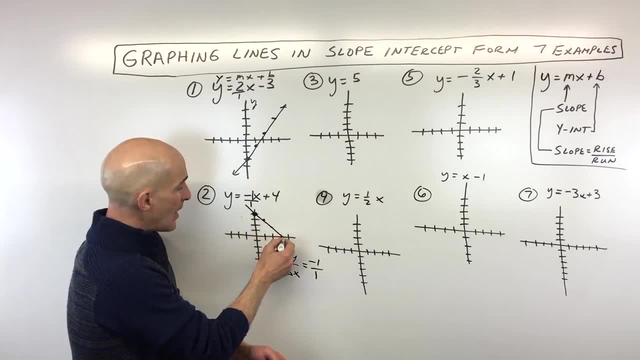 What you can check yourself is you can see that this line is going down to the right like that. okay, that tells us that it's decreasing. okay. so, just like when you read from left to right, it's going down, down, down, down. that's negative: decreasing right Going.